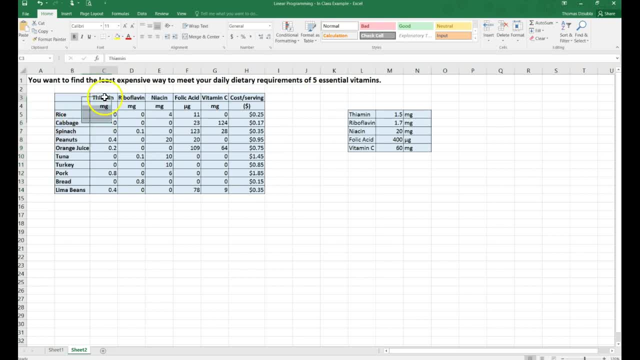 And so we have a table here of how much of these vitamins exist in each one of these. So what we're going to do is create a system of comparisons and equations that is going to calculate, based on what we would get in daily intake if we ate a certain amount or a certain number of servings of each one of these items. 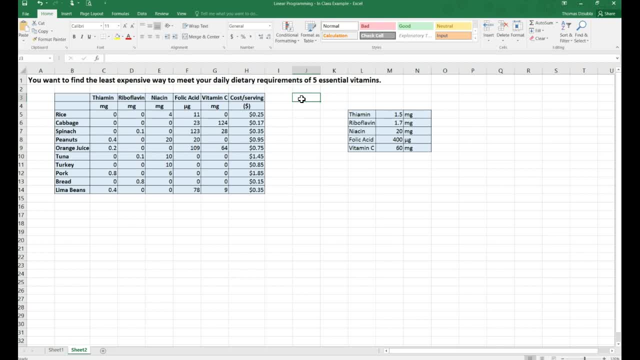 So we're going to create a new column of values of what is going to be the actual intake amount- Intake amount of Intake of food- for each one of these items here, And so we're just going to give it all a set of. 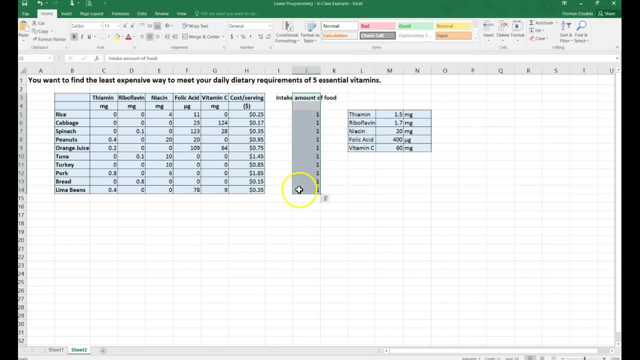 Start with a concept of one as our feed place of input. I'm going to just define it this way, just so we can have this column set up properly. Servings: Intake food Servings. So we have that Great Now in order to make this work. 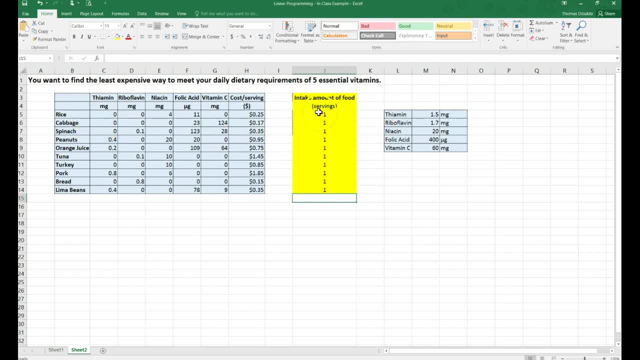 We would need to know, based on each one of these servings. if we say, take one serving of rice, that means we're going to get zero milligrams of vitamin from that, zero milligrams of riboflavin niacin. 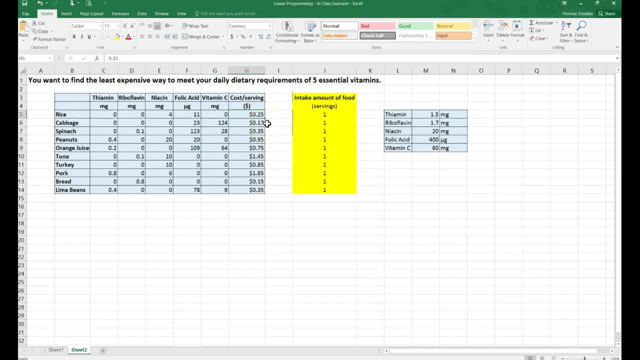 We'll get 11 micrograms of folic acid and it'll cost us a quarter per serving, So we can actually calculate out the total cost for how much we were paid for that one serving by this times this and then this times this for the folic acid. 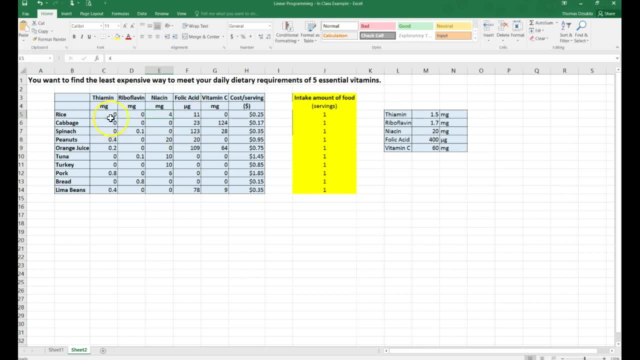 Oh, and the niacin will be. It'll be four milligrams. Now we can create a multiplication where we take each intake and multiply it by every one of these items and create a whole new table of total amount taken in and cost by food. 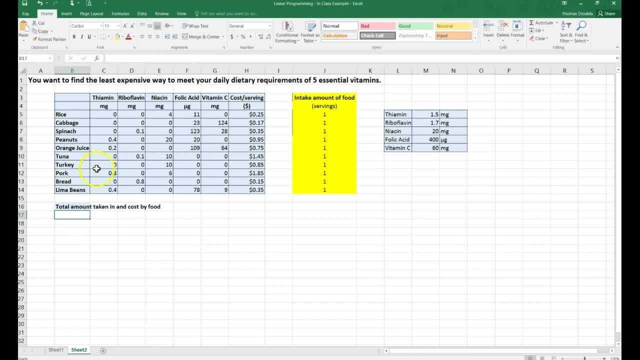 So this is going to be a new calculated table for each one of these species here- Rice and so forth, Cabbage, Penis And so forth- And we can actually copy and paste this down here and we'll just put this here. 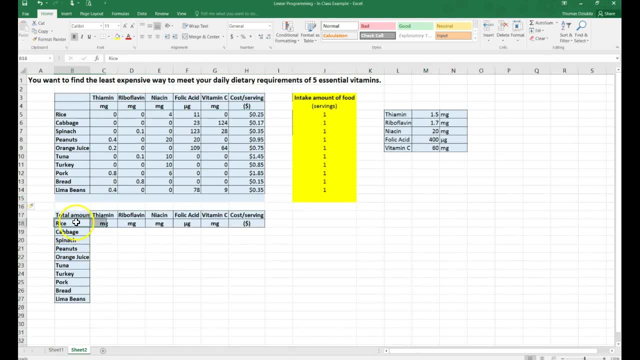 I'm actually going to give us a little bit more space. Insert: Bring this up. I'm going to change this to no fill and then I'm going to make this whole thing. Let's give this a different color, just so we can keep things straight a bit. 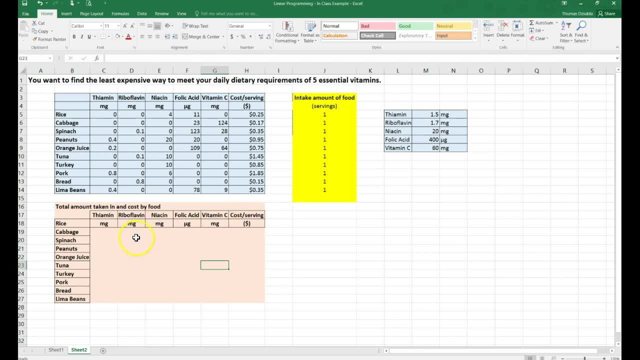 Oh, there we go. We have a new table That's going to be total intake of food, And what we're going to do is we're going to: Oops, I need to move this up, Move this up. There we go. 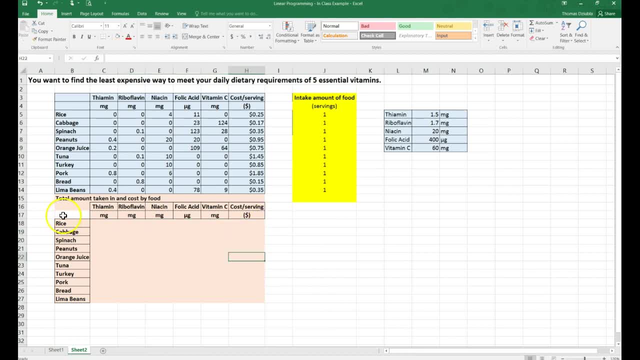 And I'm just going to copy this, so it's all the same color. And I'm going to copy this, so it's all the same color. This is just to make it pretty, Okay. So now we're going to take each one of these items and multiply every column here. 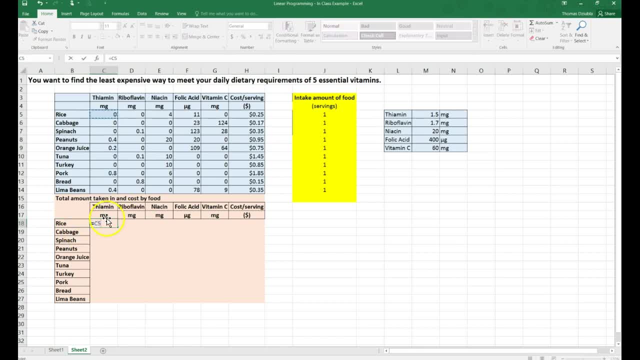 I'm going to say, Okay, This rice times this intake, And if we lock that in, I'm just going to lock it in as appropriate here, Hit enter And then just copy this across. We're going to get the total amount based on the number of servings that we're going to be changing. 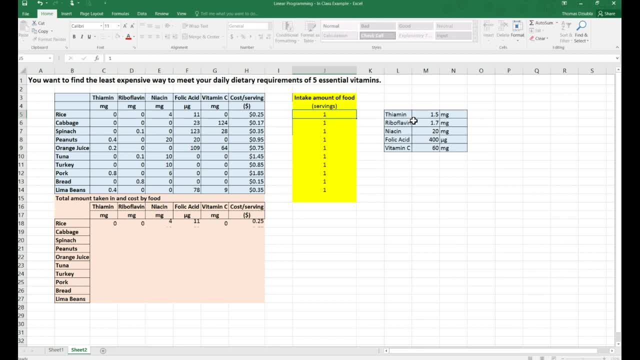 So if I was to make this a two, you'll notice it's increasing appropriately. and so forth, Or three or four. This value is going to be increasing as the total amount taken for that rice. Now if I was to just copy and paste, 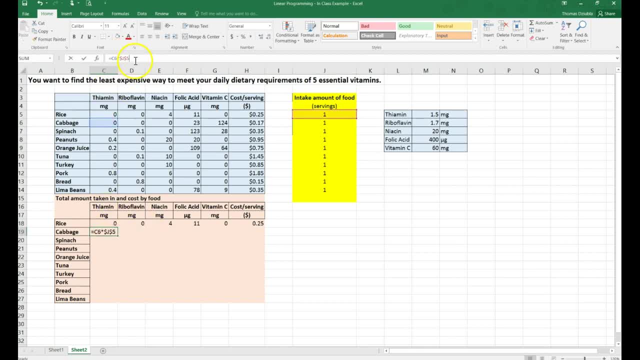 If I was to just copy and paste this down, you'll notice this won't be correct, Because here you can see this value cabbage isn't related to the total amount of cabbage that's being taken. It's still linked to rice. Why is that? 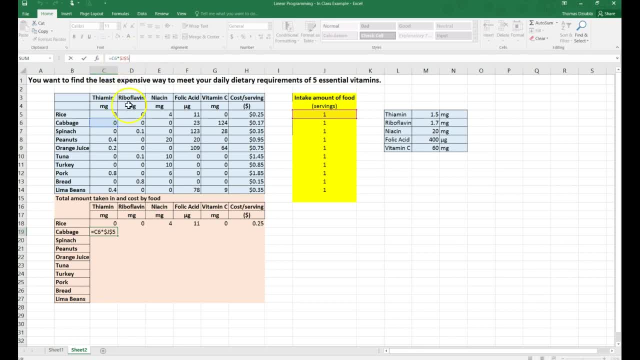 Because the absolute reference here is two dollar signs. So we can actually either manually move this down, Manually move this down And hit enter and then copy across, Or we could actually readjust this entire equation and change the formatting on this, So that here instead of saying dollar sign J, dollar sign five, we could say it's dollar sign J. 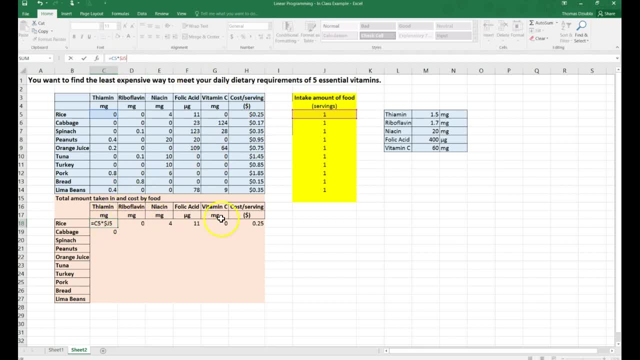 Which means it won't As I copy from left to right. it won't move the cell left to right, But if I leave five open when I copy Down the rows, this will move down with it. So it won't move this way, but it will move this way, which is exactly what we want. 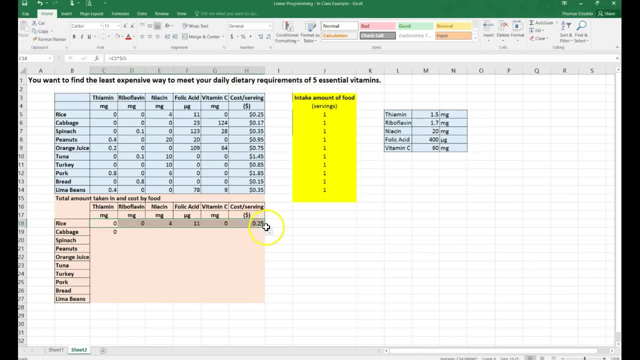 So I'm going to say: enter there, Copy across, Copy down, And we have a table now of total amounts calculated by this multiplication. So then we can say the sum of all this And this will now equal our thiamine intake. 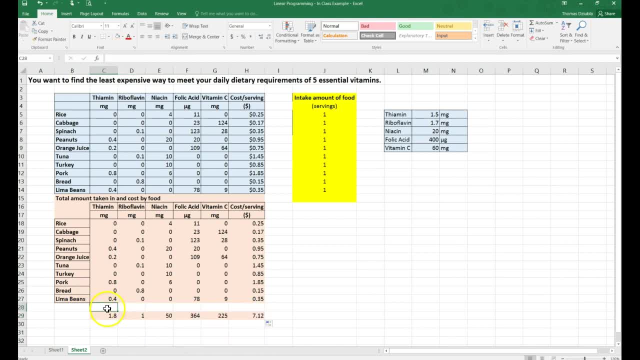 And I can copy and paste this across And this will be total amount here for all of these right. So this becomes our total amounts that we're taking in Now, if we want to go ahead and compare these totals versus these values here, which is what we want to do, 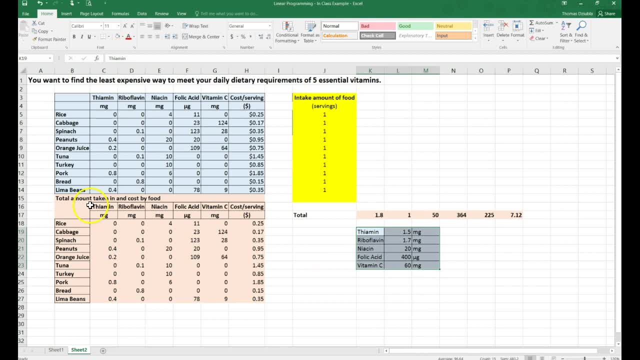 why don't we actually physically move them down in such a way that we can make sense of this? So in this case, here this first table is five, So I will place this here as thiamine. This next one is riboflavin. 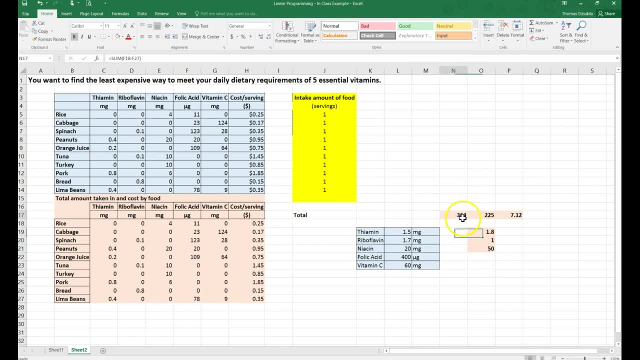 I'll make that riboflavin. This is just going down straight down the rows appropriately until we get down to vitamin C. So we just took all these totals here. I want to put that over here. And this final table here was cost servings. 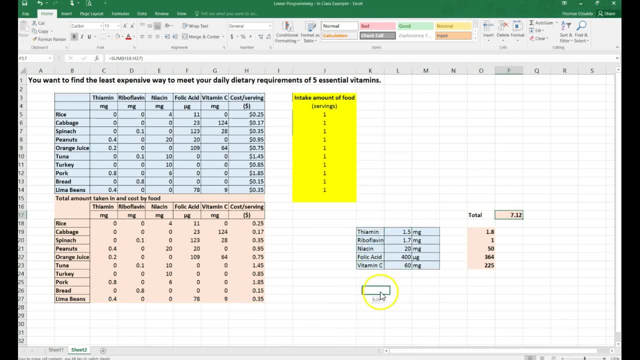 It was from this column here, So I am going to place that down here. And total cost of daily intake, And I'm going to give this a different color. Let's say this is green as the target value. So there we go. 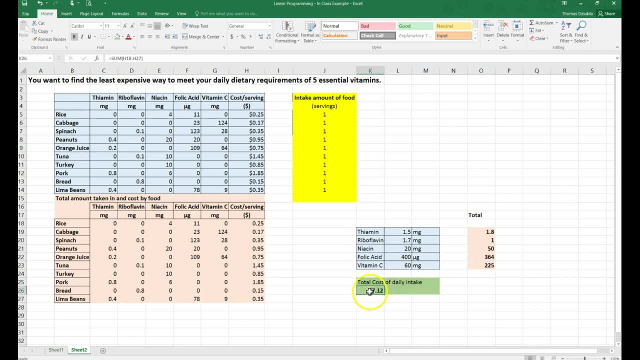 And I'll just make this whole thing green. Okay, So this is the value that we really want. I'm just going to format currency so we can know it as math, As currency, And we'll do this one as currency as well. 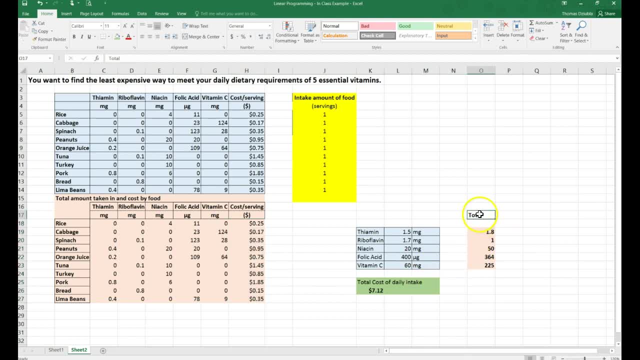 There we go, All right, So you now have this. These are the total actual intake And this is minimum requirements. Okay, So the minimum requirements is what our target is for intake. We want at least that. Another way of saying that is: 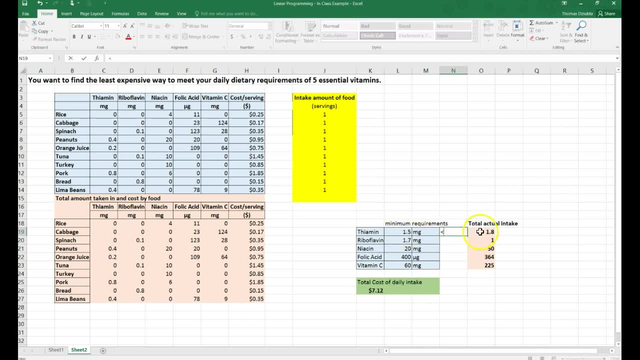 we want this value here to be less than or equal to this value. This value can be bigger, but it cannot be smaller than this one. So I'm just putting that in there for reference, so you can see the comparison we're going to make. 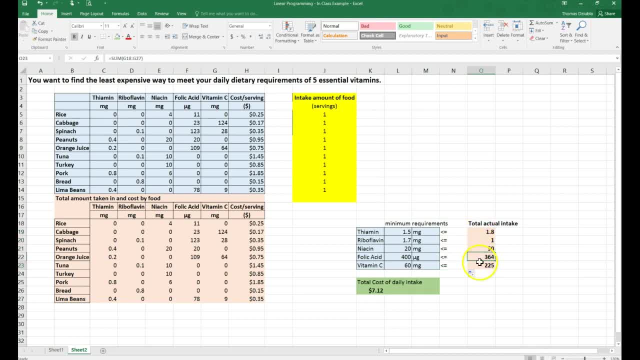 So, now that we've got this all set up, that these numbers here are actually linked to these values here, which are actually linked to these table and this input table, Same thing with this- All of these are linked values. now, Now that we have this all set up, we can actually go to our data. 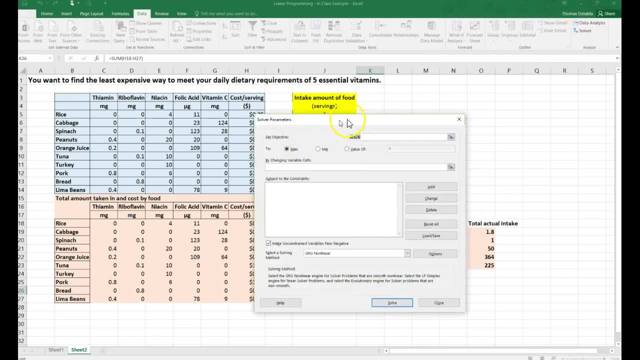 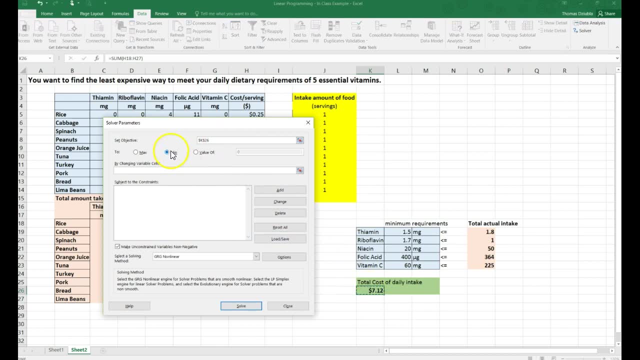 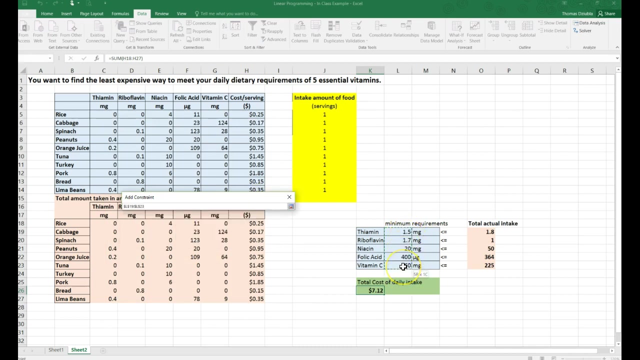 go to solver. Go to solver and specify our desire. We want to minimize. In this case, we're taking our cost. We want to minimize by changing all these intake values under certain constraints- And you can say subject to the constraints, And the constraints we're going to subject to is these values here are going. 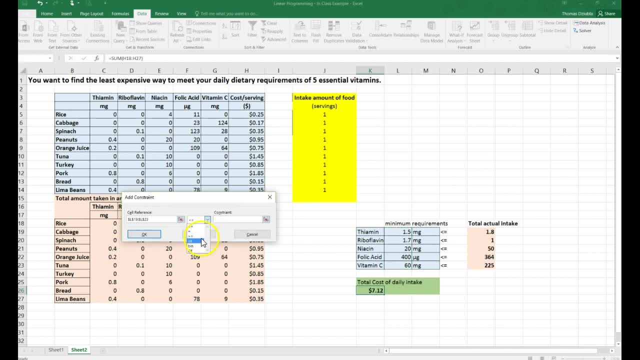 to be less than or equal to. We could make a change, We could say equal to, greater than or whatever, But in this case we just want it to be less than or equal to these columns here Let's click OK. 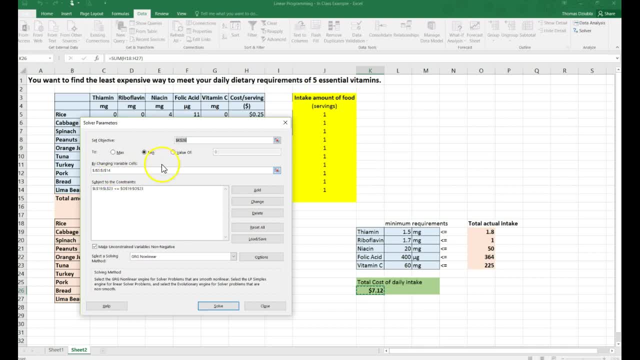 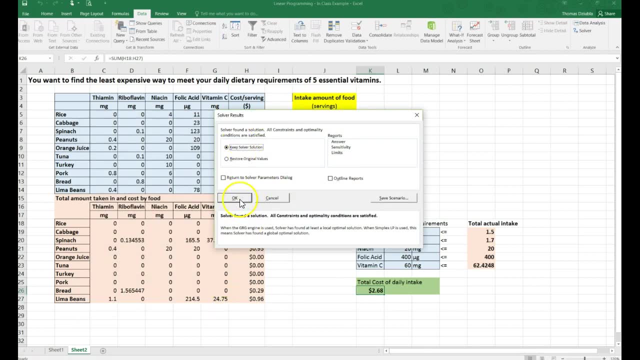 So now that we have the constraints, now that we have the cells that we're going to change, now that we have the target cell defined and we know it's minimum, click solve. It said it found its solution. We can look at it. 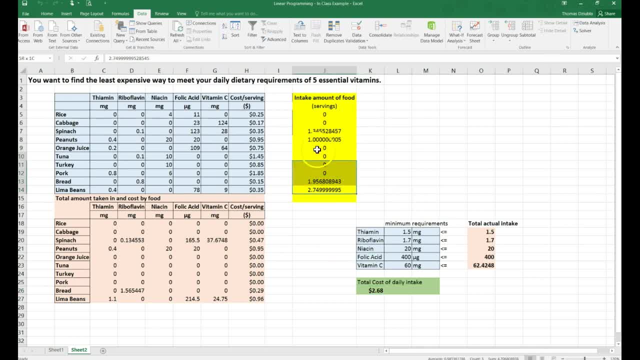 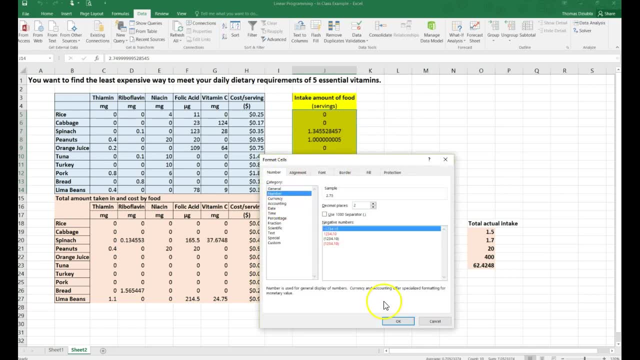 And sure enough, it found a solution for us based on the intake values. Since this is a rather large data set, we can actually change this to round it appropriately. So we'll add serving intakes And we are set up good. 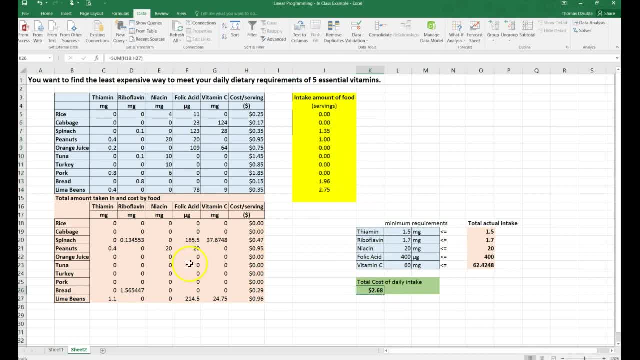 So I believe we've got a cost, We have the intake And this looks very good, All right. So now that we've got this approach done, let's attack this problem from another way, And we can do this exact same problem using a matrix math. 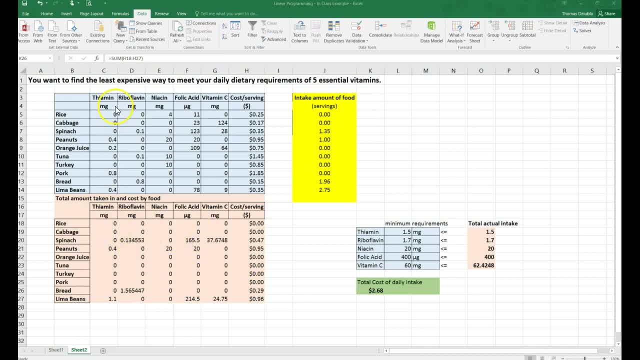 approach to solve the problem. If you notice, this is just really taking an array of data tables And instead of organizing them in two steps where we create a second table of totals, sum those totals up and reign over it, we can do it in one step using a matrix approach. 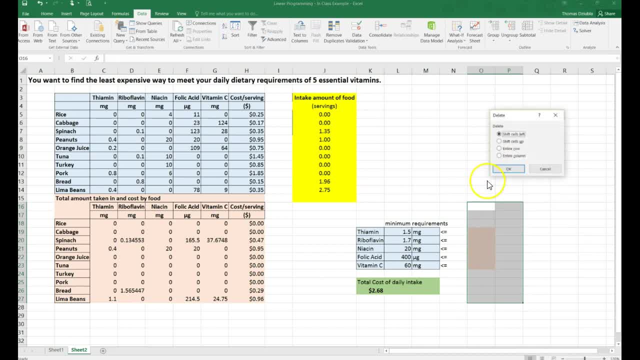 So I'm going to do that right now by just deleting all of this and resetting to 0.. Let's go back to delete, delete, let's go OK, OK And let's I'll even. I'll leave this here. 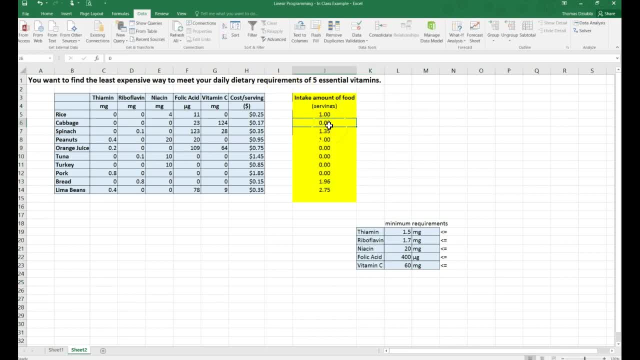 This is just our starting cells, OK, Well, no, no, no, I will. yeah, I'll leave this here, OK, So now I'll delete this too. OK, Delete, All right. So here's the starting set of problems. 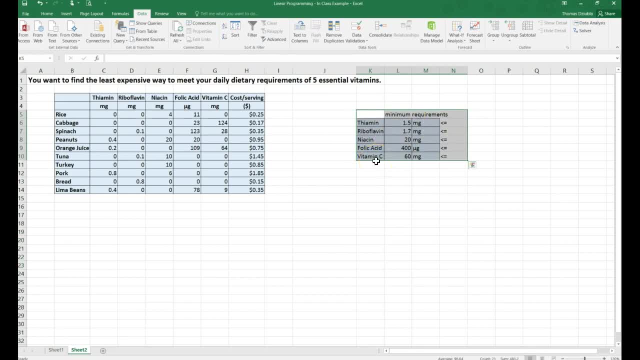 So we're going to create a. now we want to create a table of matrix approach, And in order to do that, we're going to use this cool thing called matrix of the matrix. do that is be convenient? since this is actually in the vertical column, I would 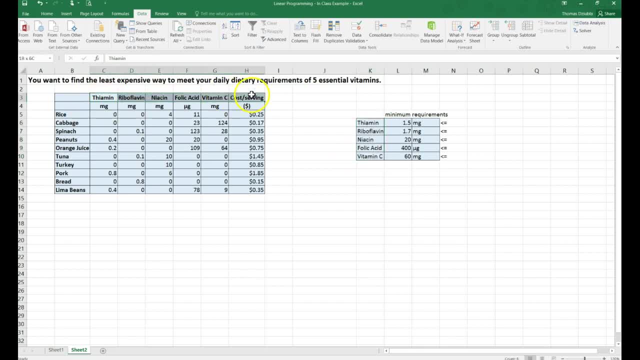 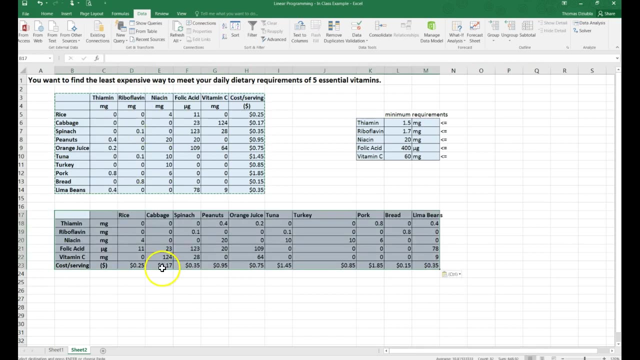 like for our table now to have all these values vertical as well. so I'm going to take this entire column table copy and I'm just going to transpose it. go to paste special and where is the transpose? transpose, oh, here, it is right there. so now we have this nice table of values where the types of food are along this: 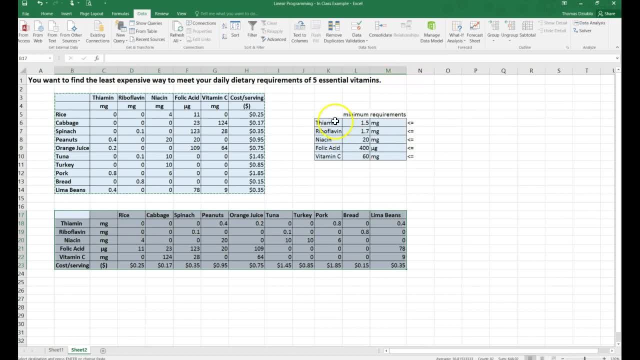 direction and all our essential minerals and so forth are in this direction. great, and so we have that. nice, now we can create a our vector and our x vector. so if we're going to put this in matrix notation, we are going to say: ax is equal to B, right? so we need to 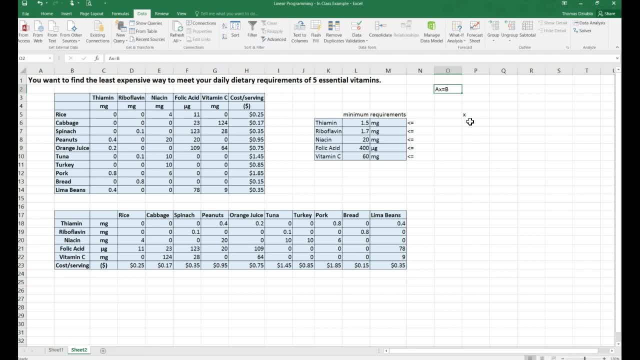 X X vector, that is our, our unknowns. in this case, it's are going to be our serving size. serving size: the size of this x vector has to be the same size of this, which is 1, 2, 3, 4, 5, 6, 7, 8, 9, 10. so we need serving size table: 1, 2, 3, 4, 5, 10. so this: 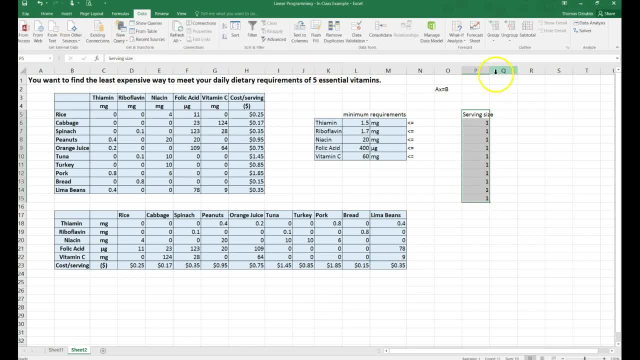 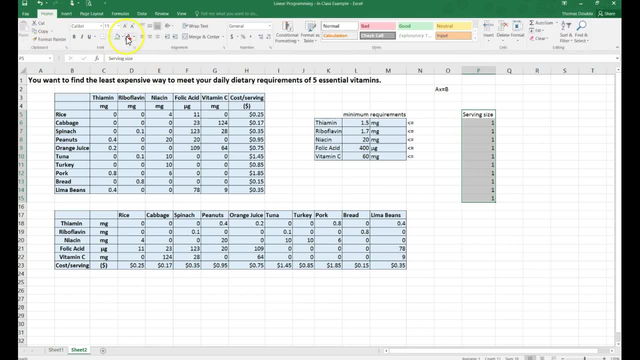 is going to be our serving size vector for our table. it's, it's home. go to fill this in as yellow and for sake of labeling, let's say copy and we'll transpose this that direction. great, and we'll fill the formatting. only I'll do should say fill formatting only there we go. so there you go. now we have two. 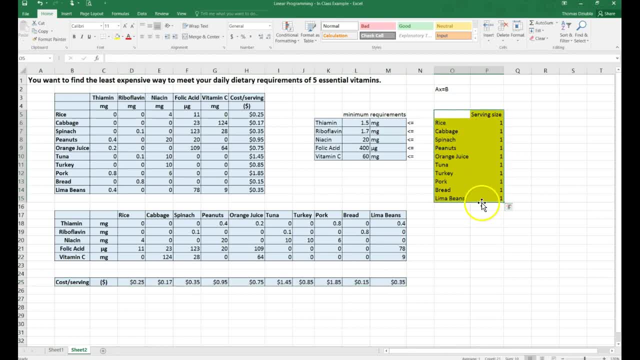 separate vectors that we're going to want to play with it. I'm just moving things around a little bit. we have a cost vector here that we're going to want to create a total cost, this total cost, and we're going to want to create a total cost and we're going to want to 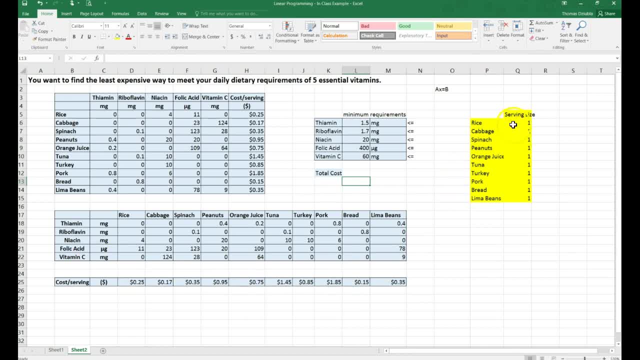 define again our cost vector for each of the three rows silicones, right? so if this is our matrix- and I'm going to start labeling these columns appropriately- this is our, this is our x vector- then I'm going to define this as our cost vector, okay, and then I'm going to define this passiert matrix, because 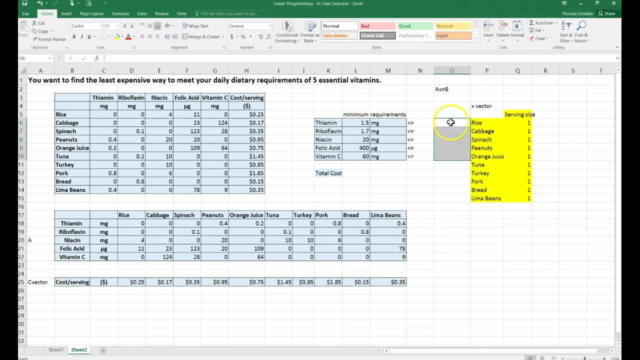 all of these other coefficients that we're going multiply by our service so I can create now our total intake as this term here AX times AXB, and this is our ideal B column. So here we just need to do malt and we're going to take the A matrix, which is this: 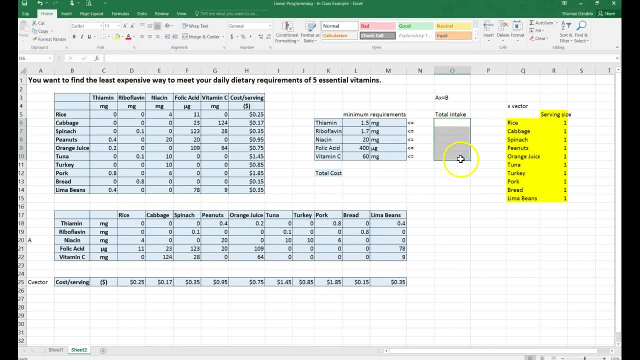 oops, yeah, select the entire range. make sure you do that. and malt. select your A matrix comma, select your appropriately matched size X matrix control shift, enter and we get that array in there. Then we can do here the same thing. it's now the cost vector times this, so this is going. 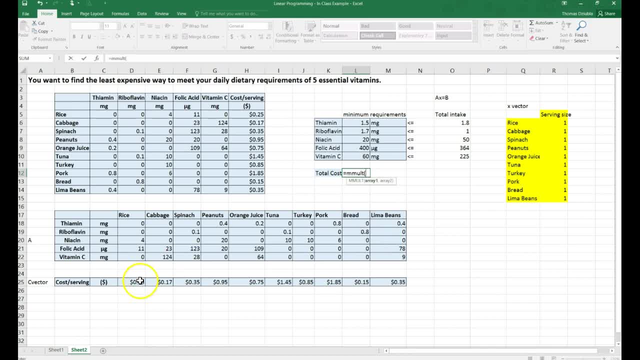 to be equal to M malt. This comma, this enter and we get the price. and I'm going to color this bold, I'm just going to format cells: currency, okay, and this is going to be okay. there we go. 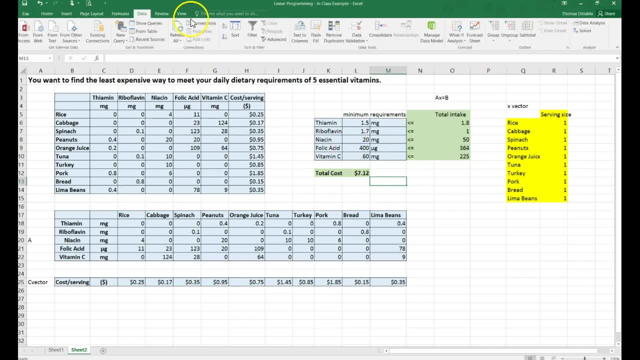 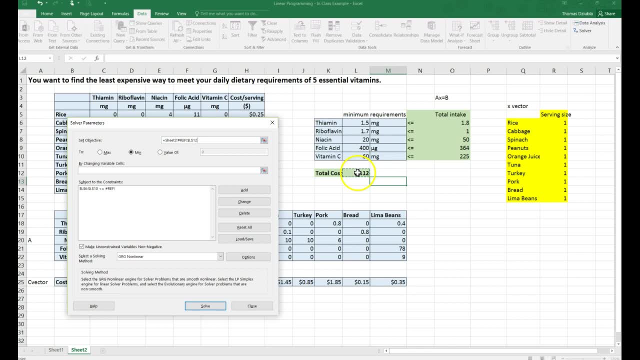 So now that we have this all set up, we're going to go ahead and create our B column. So now that we have this all set up, it's just doing the same thing we did before: Solver. okay, we go to the solver here, we tell it that we want the oops, our objective. 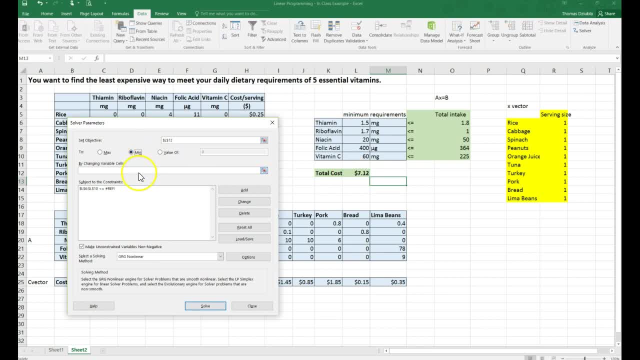 function to be the total cost. we minimize it by changing the cells. these: let's delete the prior constraint that was there, but we're going to add our constraint. our constraint is the same thing from before. All of these have to be less than or equal to. 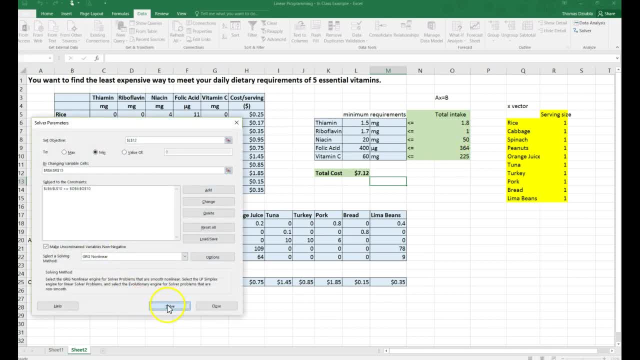 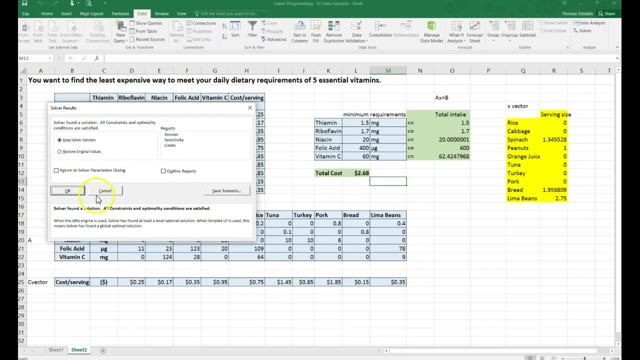 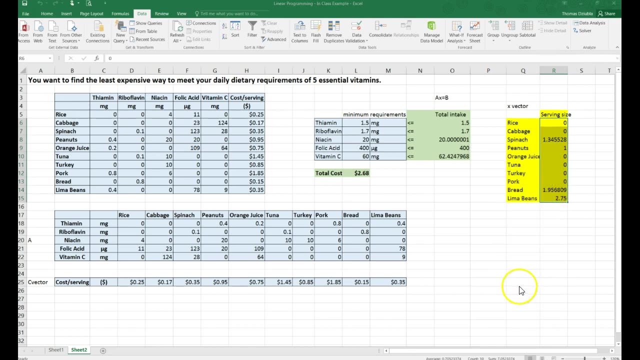 All of these okay, solve, and we get the same answer as we did before and so say okay, and here we can just go ahead and go to format cells font or number number format cells, number number. 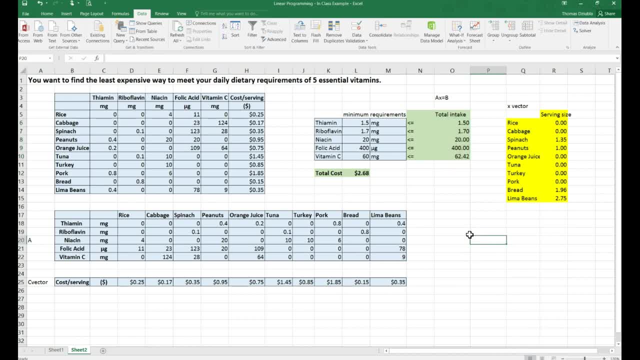 Okay, and that is, in a nutshell, how you do the. that's how you do your linear programming. It doesn't really matter at this point what it is you're optimizing. it doesn't matter whether you're doing it at cost, total intake time, as long as you have some value that. 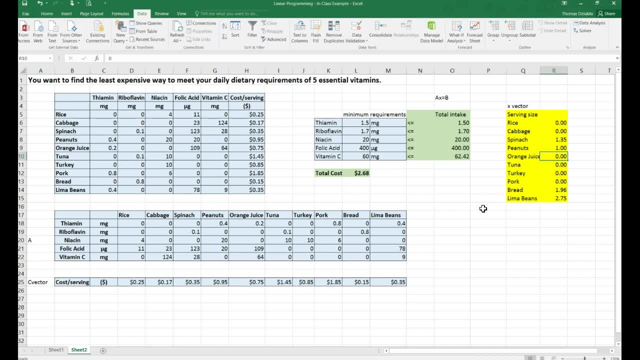 you're going to minimize or maximize and you have constraints of other variables that you're trying to work within. If you can set up a series of linear equations to describe that, you can use linear programming to find an optimum value for your solution, and this is exactly how you do it. 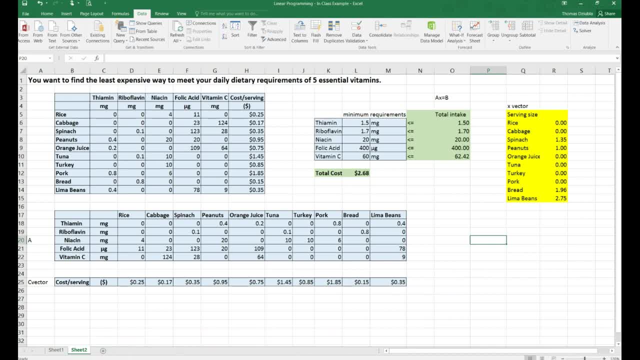 So hopefully this makes sense and I will now go on to macros. Thanks a lot.